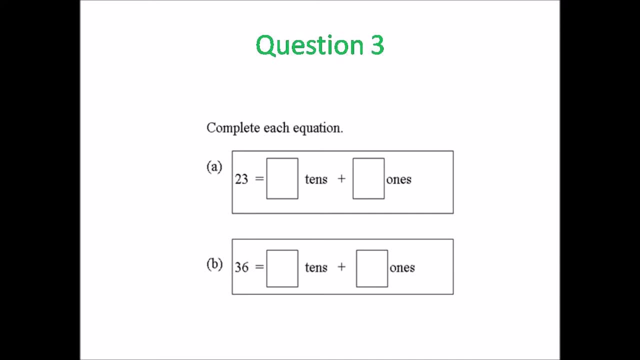 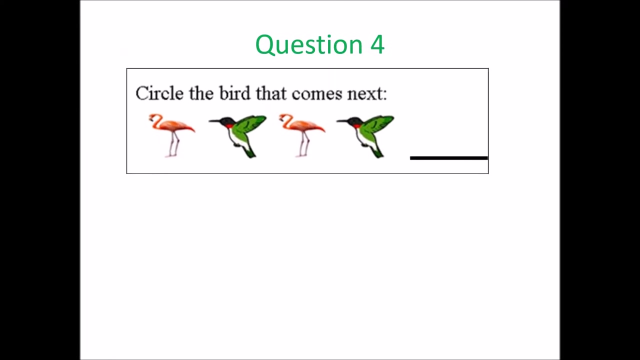 tens plus how many ones. Do that? first? Put a number for the tens, Put a number for the ones, And 36 is equal to how many tens and how many ones. So just put your numbers in the boxes. Got it? Question four: Circle the bird that comes next And you have. 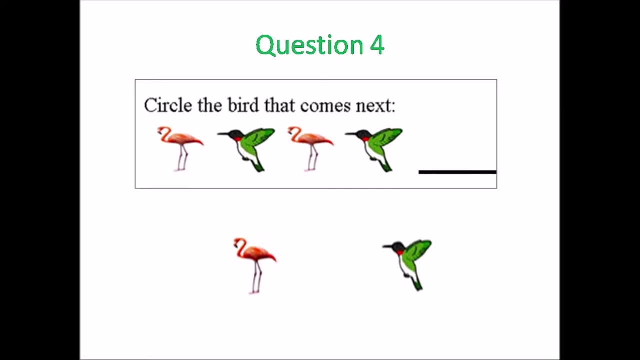 flamingo hummingbird. Flamingo hummingbird, what bird would come next, given that pattern? circle it and we will move on to question five. complete this addition: fact family. so remember what a fact family is. and you have the numbers two, one and three that comprise this, that make up this fact family. two plus one is three, right? 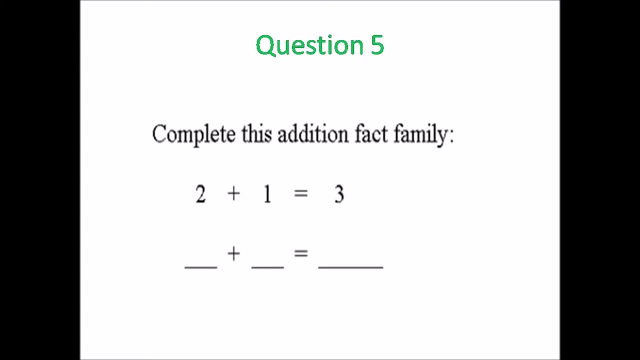 another fact, addition fact for that: two plus one is three and we move on to question six. ray has three marbles. he won four more marbles. how many marbles does ray have all together? so it's a word problem that you have to solve. remember you can put sticks. 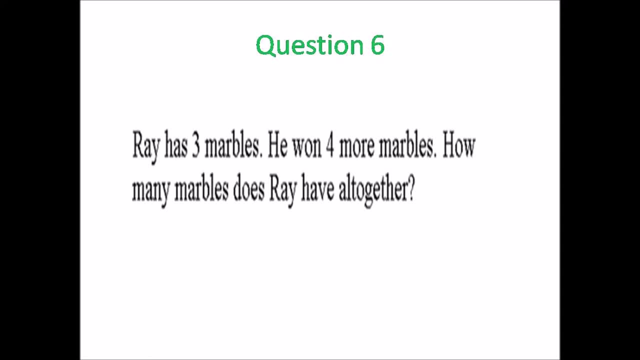 or circles represent the marbles. add them up and see how many ray would have all together. question seven: compare these numbers using those symbols. those symbols would be less than, greater than or equal to, and you're comparing the numbers eight and five. use one of those symbols to compare the numbers eight and five. 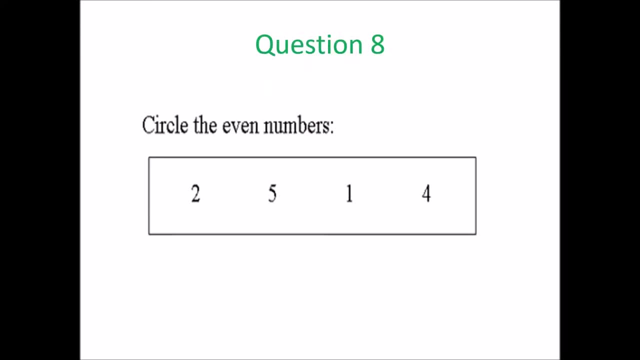 question eight: circle the even numbers. look at the numbers that are given: two, five, one and four. circle all of the even numbers. go ahead, just circle the even numbers. got it. question nine: circle the shape that comes next in this pattern. circle the shape that comes next six. 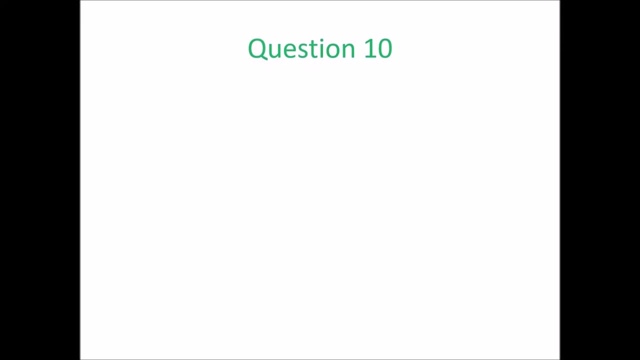 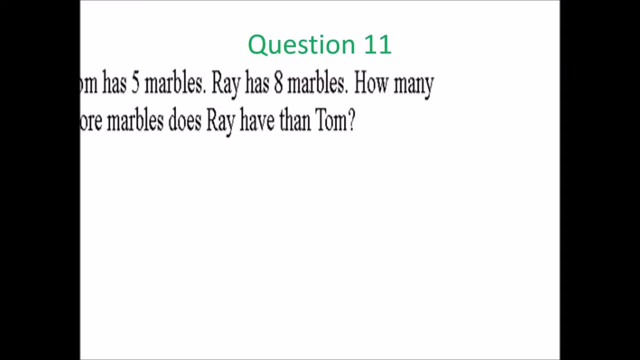 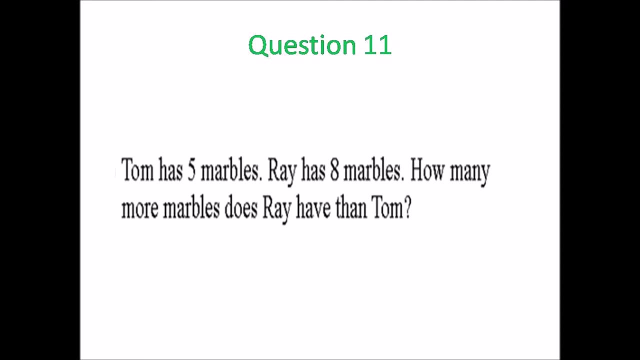 question 11: word problem: tom has five marbles. ray has eight marbles. how many more marbles does ray have than tom? tom has five marbles. ray has eight marbles. how many more marbles does ray have than tom? so do the working come up with an answer? 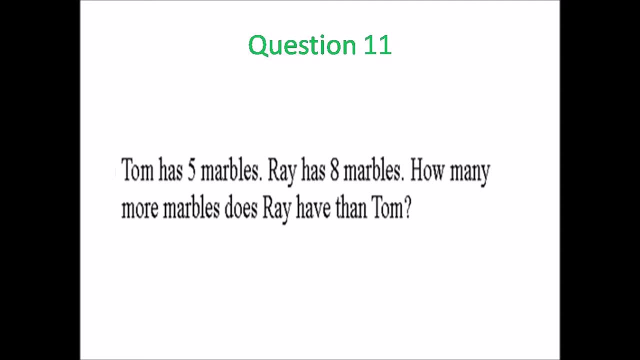 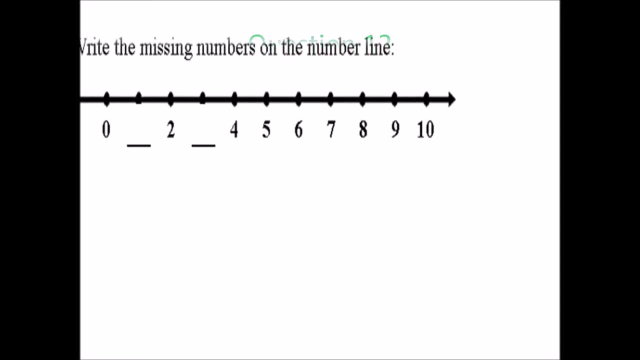 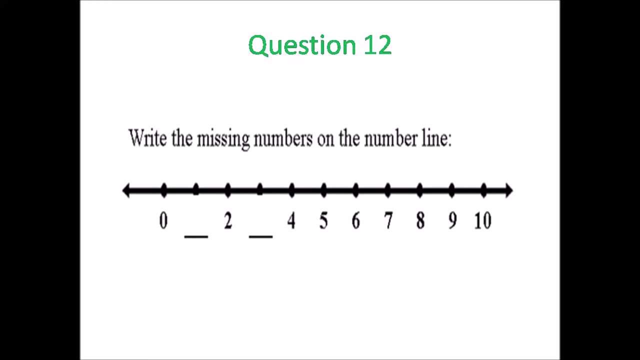 another word problem and we move on to question 12.. write the missing numbers on the number line. there are two numbers that are missing on that number line. write those two numbers that are missing on the number line, number 13.. complete this subtraction fact: family seven take away five equals two. so write another equation for that. 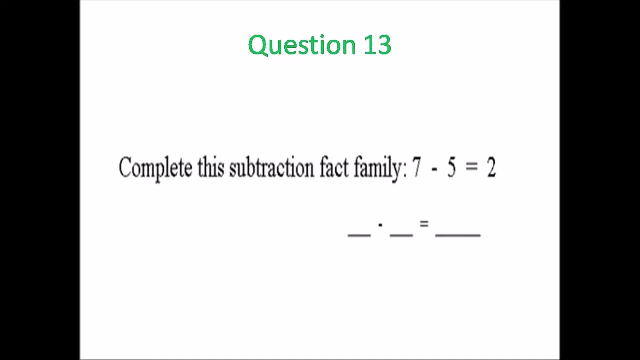 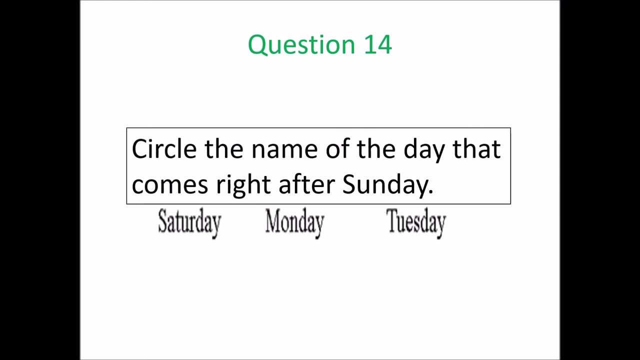 subtraction fact: family. remember you have to use the same numbers because the numbers are family. seven take away five is equal to two number 14.. there we go. circle the name of the day that comes right after sunday. circle the name of the day that comes right after sunday. is it saturday or monday or tuesday? circle one of those days. 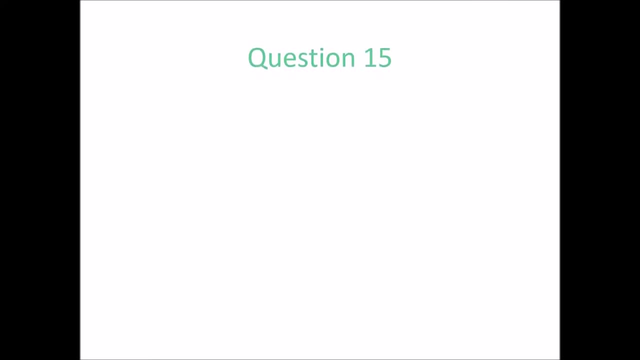 got it and we move on now to question 15.. six plus three is equal to what? so you're doing horizontal addition. six plus three is equal to something. do it on your fingers or put sticks or circles. six plus three- what do you get? just go to six plus three. 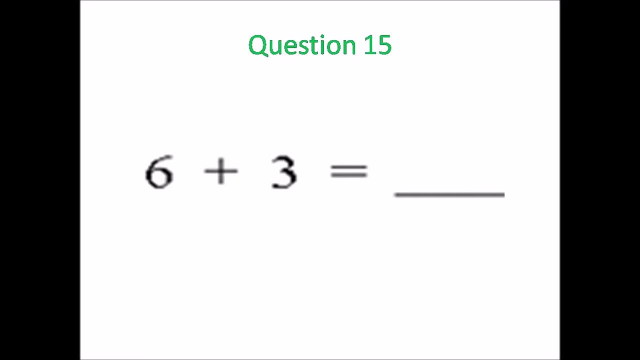 six and count on three from six, question 16.. here we go. arrange these numbers in descending order. you have to know descending order, what that means. arrange these numbers in descending order, and the numbers are five, ten, two, 15 and one. write them in descending order. do it quickly before we move on. 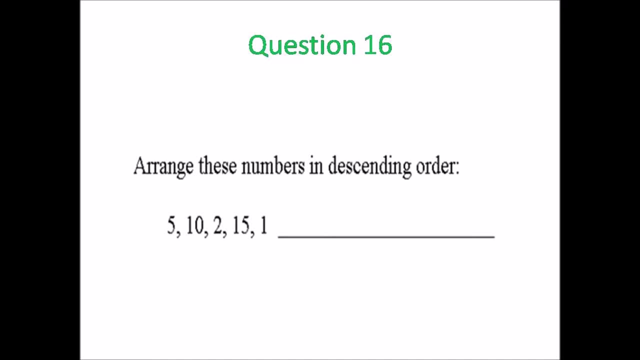 17.. so we got it excellent work. one open question, no two, we can't careful. 17, 10 take away four is equal to 4.. so you have horizontal subtraction. now, ten take away 4 is equal to what? so you have to work yarn values, whatever. 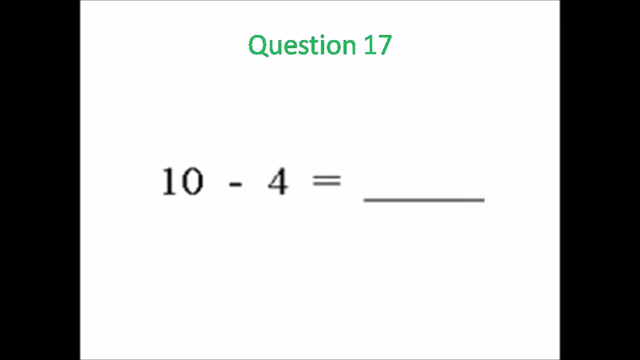 16: right, you have 10 fingers so you can easily do it: put up 10 fingers and take away four. see what you're left with: 10, take away four. this is basic stuff for grade two. question 18 now. circle the name of the month that comes right before March. circle the name of: 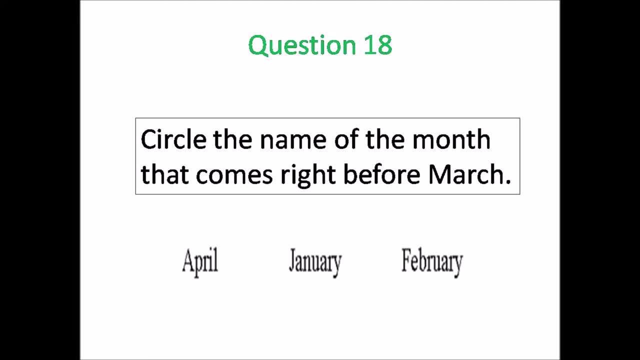 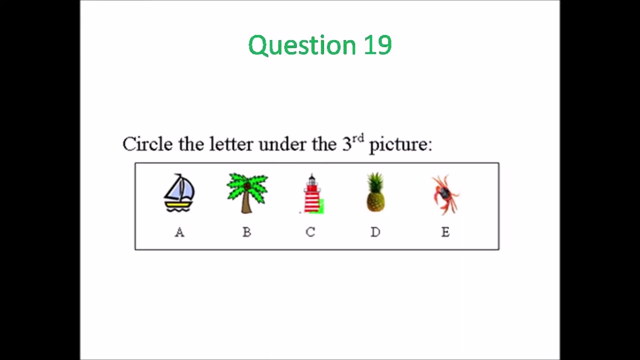 the month that comes right before March. is it April, January or February? circle: the name of the month that comes right before March and we move on to question 19. circle: the letter under the third picture. circle: the letter under the third picture. so is it a, B, C, D or E? you look at the pictures you want to. 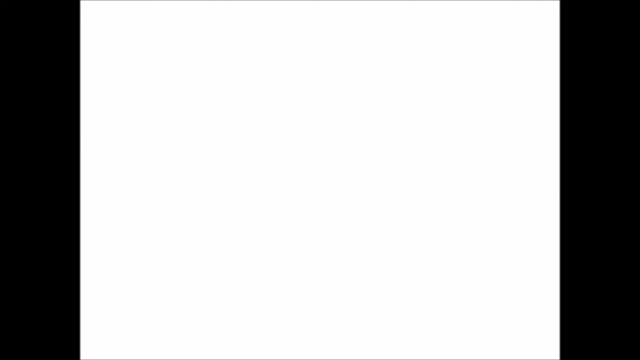 circle the lead under the third picture. question 20: circle: the solid shape. there are four shapes. one of them represents a solid shape circle, the one that shows the solid shape. question 21: 74 plus 12. 74 plus 12. so you're doing vertical addition now. so 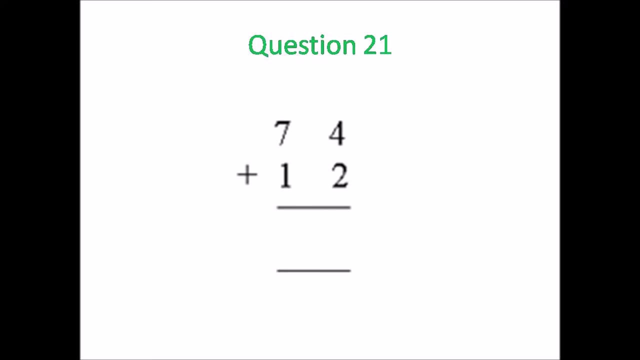 you can do these on your fingers or put sticks or circles. 74 plus 12. and we move on to question 22: circle the cylinder. four shapes are there. one of them represents a cylinder. circle the cylinder. question 23: write the numeral 602. remember, numeral and number same thing. write the number or write the numeral 602. 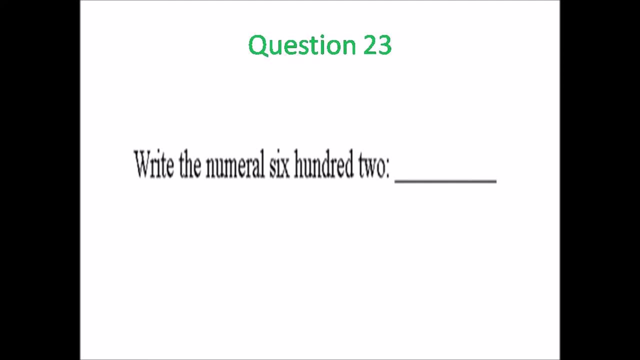 oh, got it. question 24: circle the object that is shaped like a rectangular prism. some big words, O here, O ere, And you have four objects there. Which one is shaped like a rectangular prism? Let's go grade two, Question 25.. Shade two quarters of this shape. 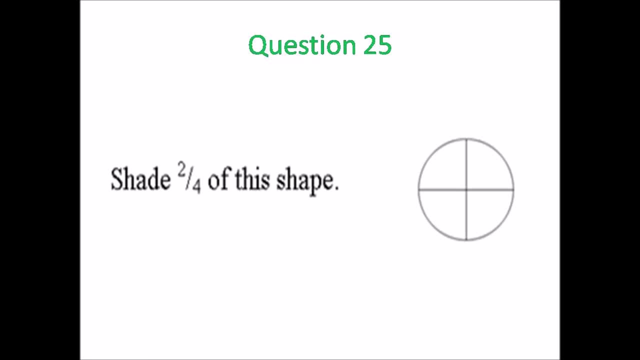 Shade two quarters of this shape. Just divide it into quarters. Shade two quarters of the shape. Shade two quarters of this shape, Got it Good. Question 26.. What time is it? look at the clock face. What time is it. 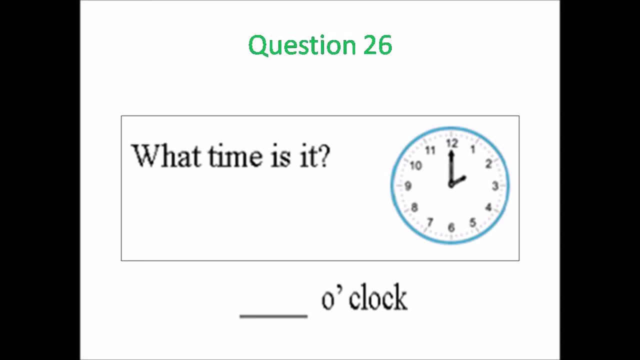 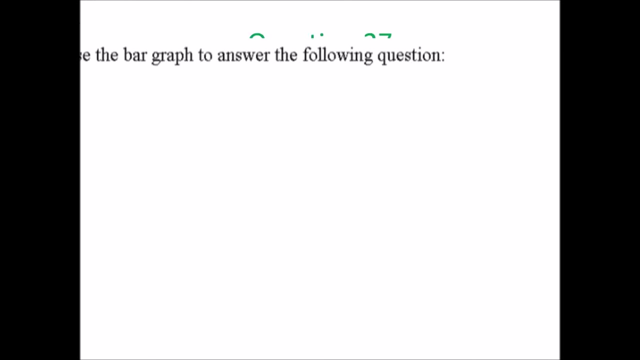 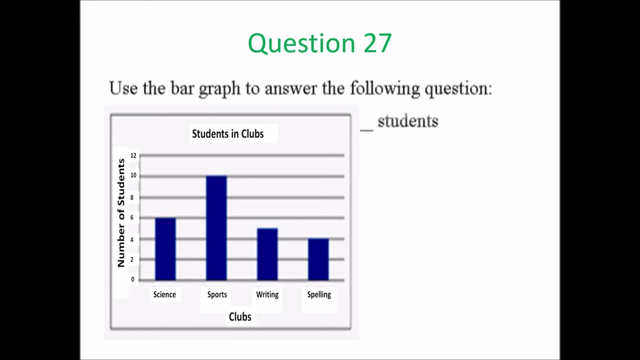 It's something o'clock. let's go great to know you can get that correct and we move right along to question 27. let's go great to use the bar graph to answer the following question. and there is the bar graph: students and clubs- number of students. 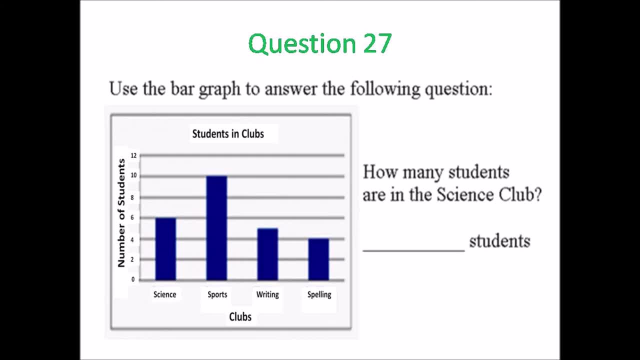 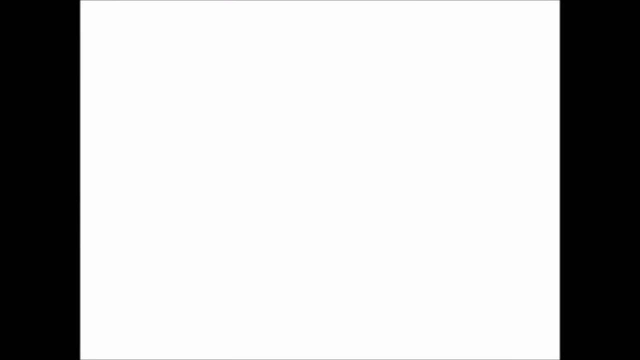 and the clubs: science, sports, writing, spelling. how many students are in the science club? how many students are in the science club? done, yes, we move on to question 20. question 20. question 20: eight circle: the letter which the spinner. eight circle: the letter which the spinner. 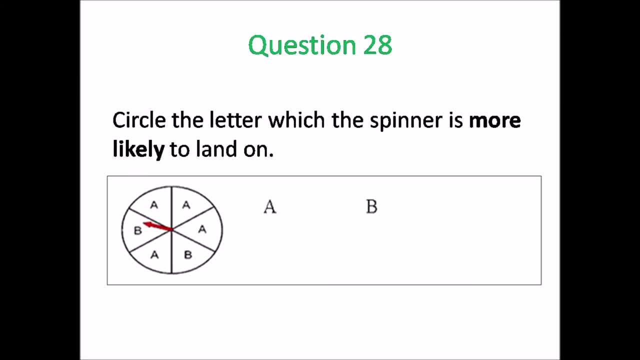 eight: circle: the letter which the spinner is more likely to land on circle. the is more likely to land on circle. the is more likely to land on circle the letter which the spinner is more likely. letter which the spinner is more likely. letter which the spinner is more likely to land on. 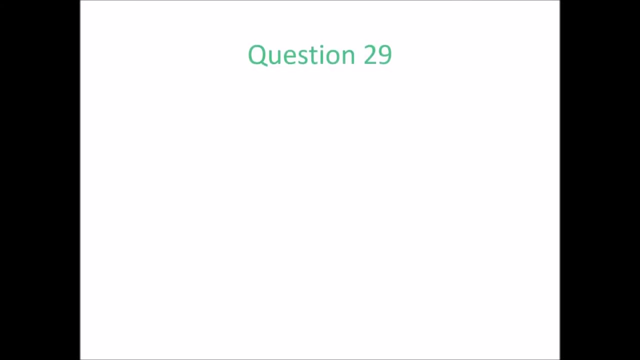 question 29. question 29. question 29: 96. take away 53. 96. take away 53. 96. take away 53. so you're doing vertical subtraction. so you're doing vertical subtraction, so you're doing vertical subtraction. 96. take away 53. use your fingers or use. 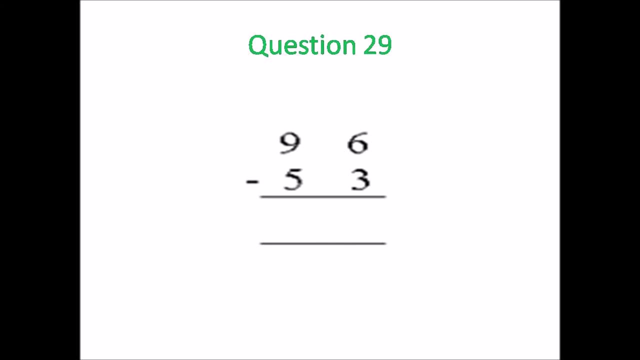 96- take away 53. use your fingers or use 96- take away 53. use your fingers. or use circles or sticks to work it out. circles or sticks to work it out. circles or sticks to work it out. do it quickly. do it quickly. do it quickly. 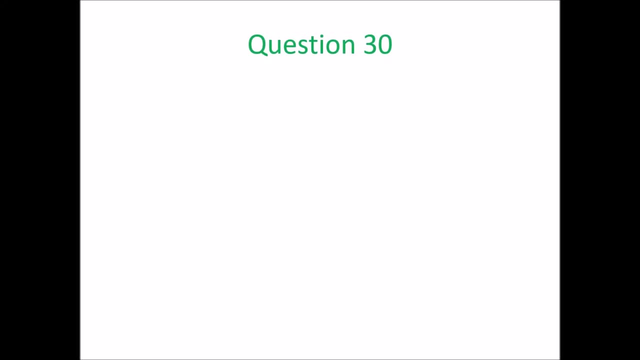 no regrouping or renaming. so you're no regrouping or renaming. so you're no regrouping or renaming. so you're straight, straightforward, straight, straightforward, straight, straightforward. question 30: all of the following shapes: question 30: all of the following shapes: question 30: all of the following shapes are made up of squares. 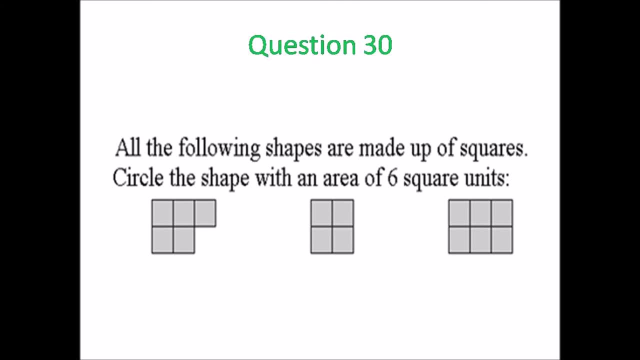 are made up of. squares are made up of squares: circle, the shape with an area of six. circle, the shape with an area of six. circle, the shape with an area of six square units. square units, square units: three shapes there which one has an area. three shapes there which one has an area. 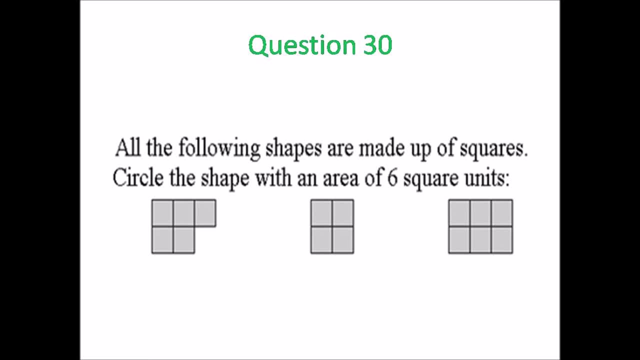 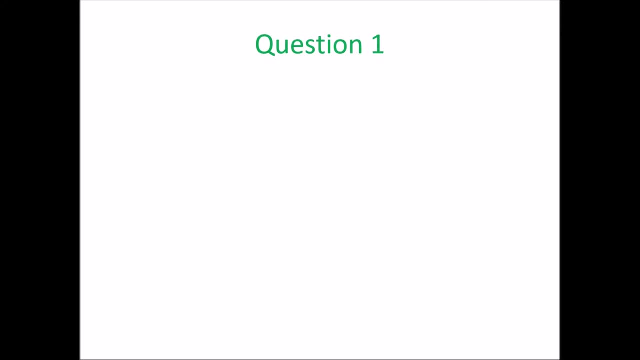 now the fun part. you will mark your answers. here we go question one. what was answers? here we go question one. what was answers? here we go question one: what was the answer to question one? the answer to question one. the answer to question one. write the number at the place value. 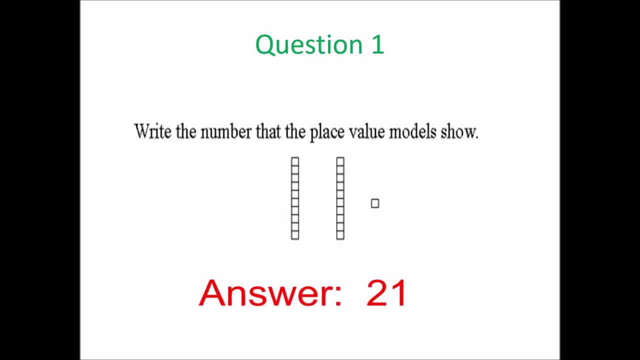 write the number at the place value. write the number at the place value. model show- model show. model show: it's a two digit number. yes, that it's a two digit number. yes that it's a two digit number. yes, that number is 21: two tens and one one. 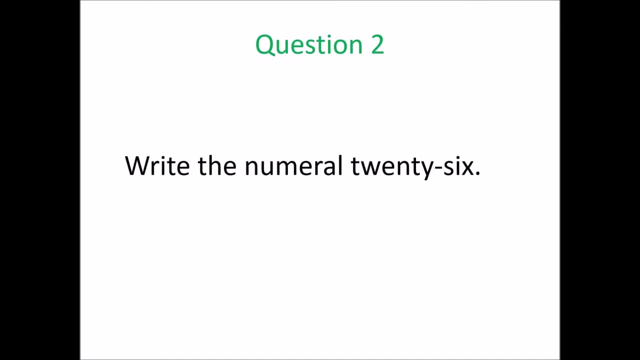 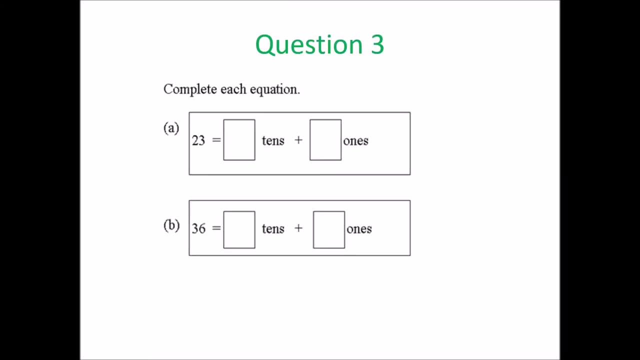 write it using numbers: 26 is 2 6- 26. write it using numbers 26 is 2 6- 26. got it. question three: got it. question three. got it. question three: complete each equation: yes, the first one. complete each equation: yes, the first one. 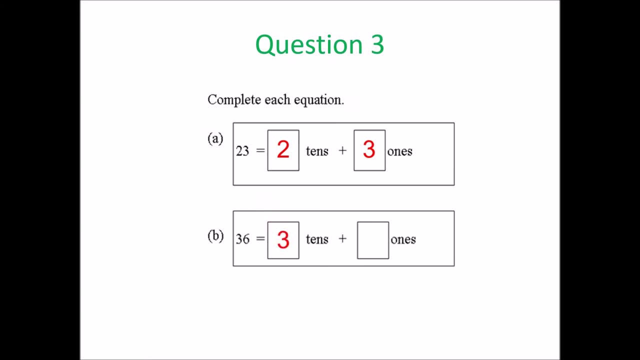 complete each equation. yes, the first one is 223, so it's two tens and three ones is 223, so it's two tens and three ones is 223, so it's two tens and three ones. and then it's three tens and six ones, and then it's three tens and six ones. 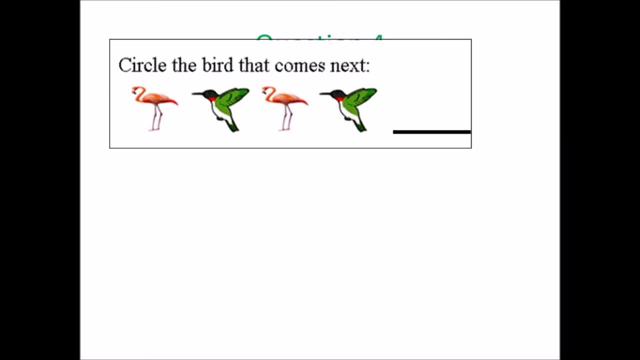 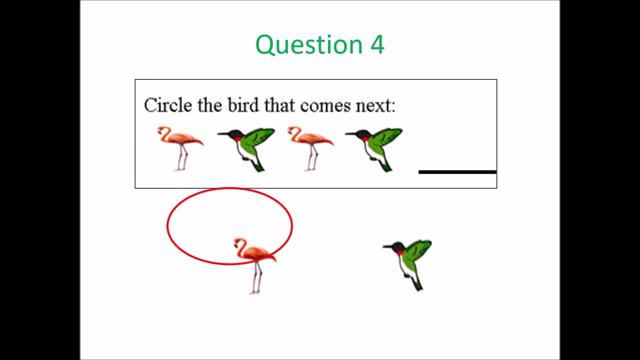 and then it's three tens and six ones. question four, question four. question four: circle the bird that comes next. circle the bird that comes next. circle the bird that comes next. here we go circle it. yes, the flamingo, here we go circle it. yes, the flamingo. 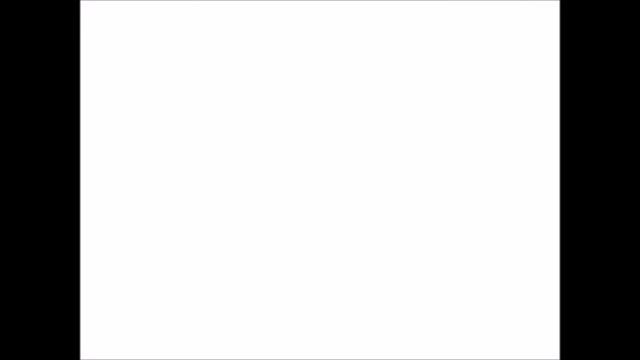 here we go, circle it. yes, the flamingo would come next, would come next, would come next. question five, question five. question five: complete this addition fact: family two. complete this addition fact: family two. complete this addition fact: family two plus one is three plus one is three plus one is three. so use the same numbers, one plus two. 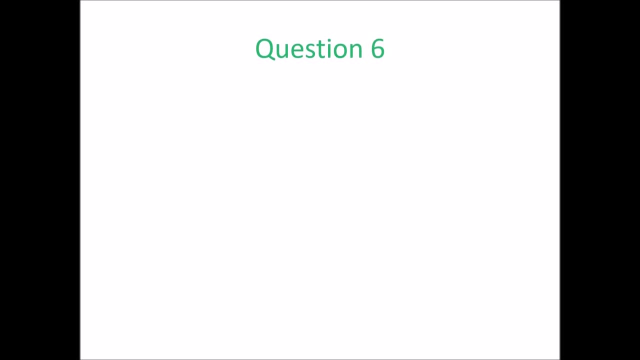 so use the same numbers. one plus two. so use the same numbers. one plus two is three, is three, is three. question six, question six. question six: raise three marbles, he won four more. raise three marbles, he won four more. raise three marbles, he won four more marbles. how many marbles does ray have? 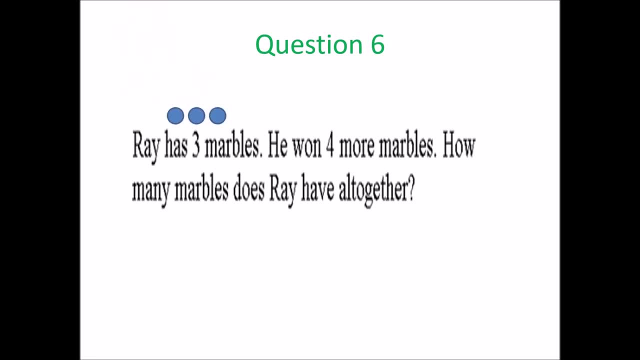 marbles. how many marbles does ray have marbles? how many marbles does ray have all together? put three marbles above all together. put three marbles above all together. put three marbles above three, but four marbles above four. three but four marbles above four. 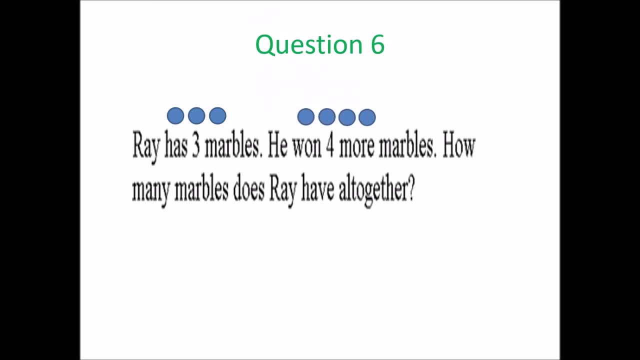 three, but four marbles above four. count them up: one, two, three, four, five. count them up: one, two, three, four, five. count them up: one, two, three, four, five, six, seven, six, seven, six, seven, three would have seven marbles. question seven. question seven. question seven. compare these numbers using the symbols. 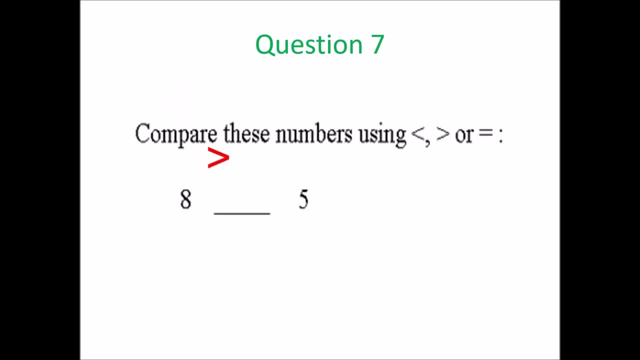 compare these numbers using the symbols. compare these numbers using the symbols: eight and five. so you have to point it: eight and five. so you have to point it: eight and five. so you have to point it to the five. so eight is greater than to the five. so eight is greater than. 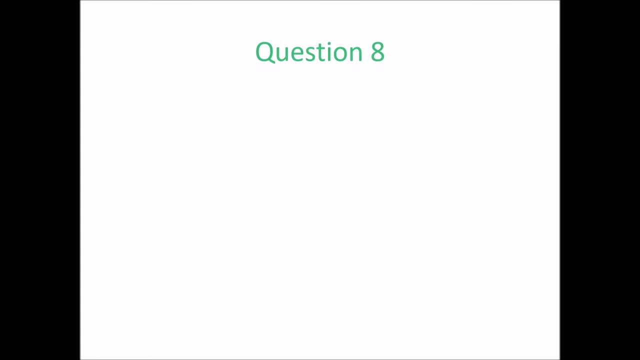 to the five. so eight is greater than five. question eight: circle even numbers. let's circle them. circle even numbers, let's circle them. circle even numbers, let's circle them. yeah, two is even. yeah, two is even. yeah, two is even. circle the next one? wait on it. 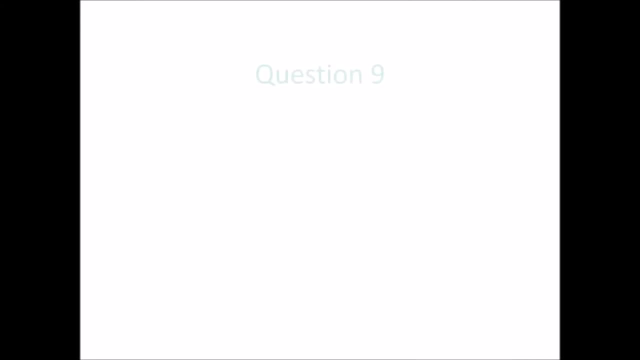 circle the next one, wait on it. circle the next one, wait on it. four, four, four, two and four, even numbers. two and four, even numbers. two and four even numbers. question nine, question nine. question nine: circle the shape that comes next circle. the shape that comes next circle. the shape that comes next circle it. let's go circle it. 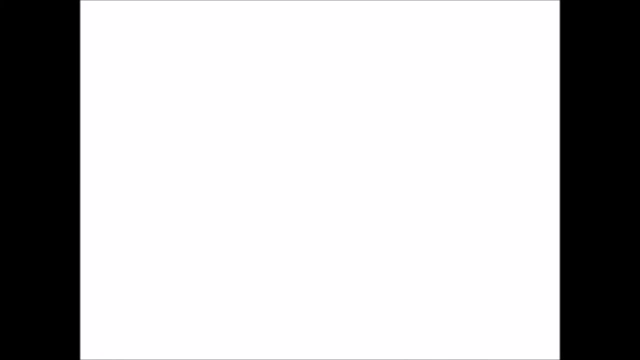 circle it, let's go circle it, circle it, let's go circle it. here the circle would come next. very here the circle would come next, very here the circle would come next. very good. question 10: what comes next? two, four, six, eight, ten? what comes next? two, four, six, eight, ten? 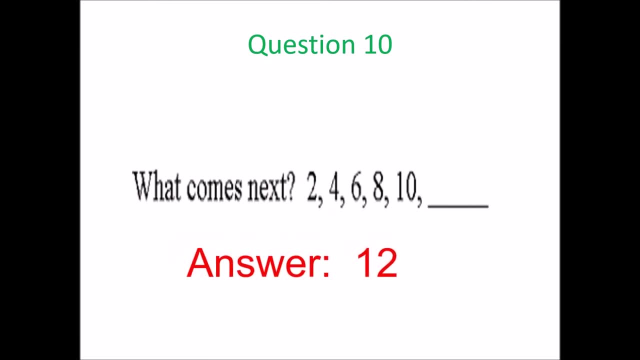 what comes next? two, four, six, eight, ten. what number would come next? wait on it. what number would come next? wait on it. what number would come next? wait on it. wait on it. there it is 12, you're. wait on it. there it is 12, you're. 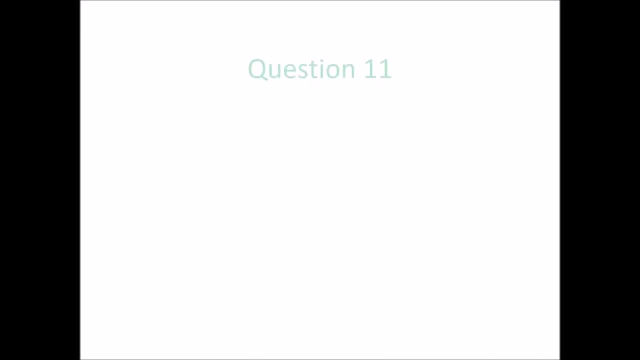 wait on it. there it is 12. you're counting up by twos, going into counting up by twos, going into counting up by twos, going into skip counting by two, skip counting by two, skip counting by two. question 11: raise five: marbles thomas, five raise. 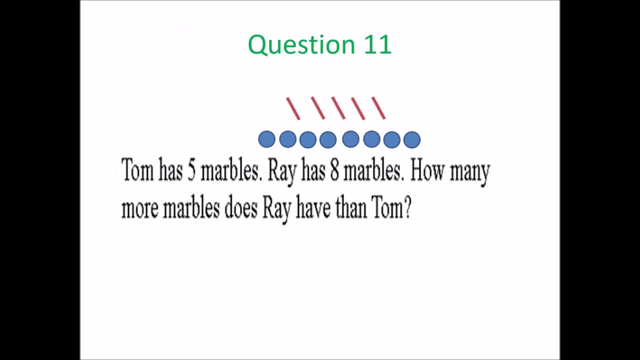 raise five marbles thomas, five raise. raise five marbles thomas, five raise eight. how many marbles is rehab? how many, eight? how many marbles is rehab? how many, eight. how many marbles is rehab? how many more houses we have than tom take away? 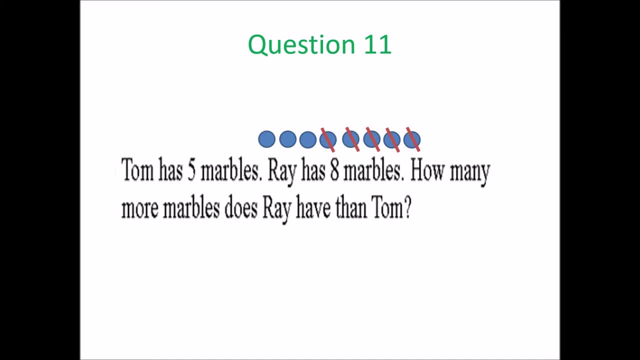 more houses we have than tom take away. more houses we have than tom take away. five from the eight one, two, three, five from the eight one, two, three, five from the eight one, two, three. so we would have three more marbles than so. we would have three more marbles than. 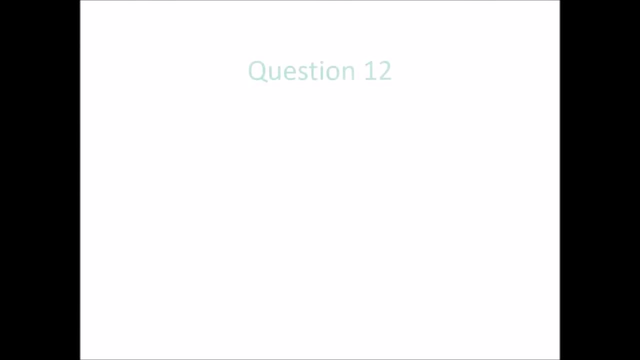 so we would have three more marbles than tom. question 12.. write the missing numbers on the number. write the missing numbers on the number. write the missing numbers on the number. line what two numbers are missing, but line what two numbers are missing, but line what two numbers are missing, but i'm in: yes, one. what else is missing? 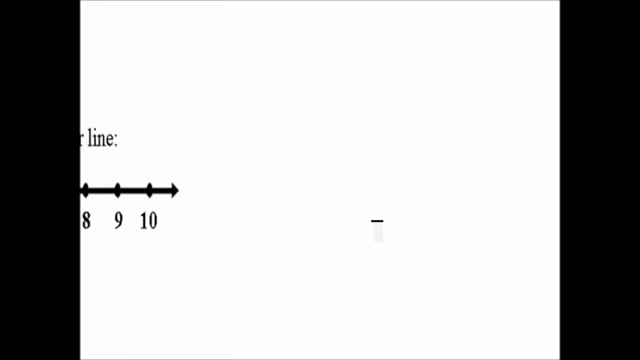 i'm in: yes, one. what else is missing? i'm in: yes, one. what else is missing? zero, one, two, three, one and three. question 13.. complete this subtraction fact family. complete this subtraction fact family. complete this subtraction fact family seven. take away five is two, so seven. 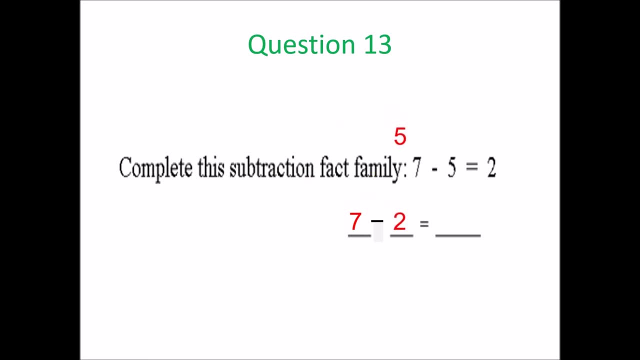 seven take away five is two, so seven- seven take away five is two, so seven take away two is take away two is take away two is five. yeah, use the same numbers, just five. yeah, use the same numbers, just five. yeah, use the same numbers, just switch them around. 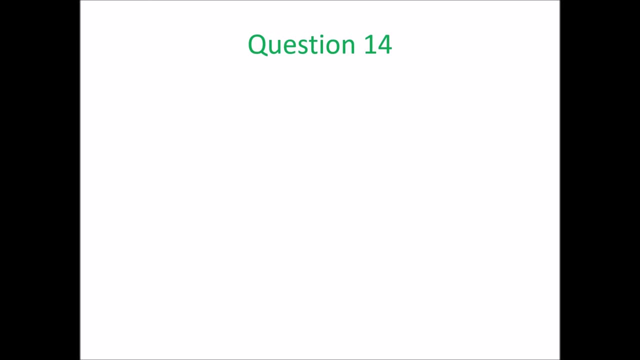 question 14.. circle: the name of the circle, the name of the circle, the name of the data comes right after sunday. data comes right after sunday. data comes right after sunday. which one is it wait on it? wait on it. which one is it wait on it? wait on it. 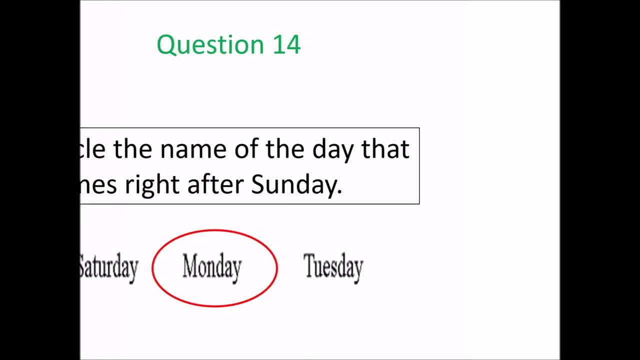 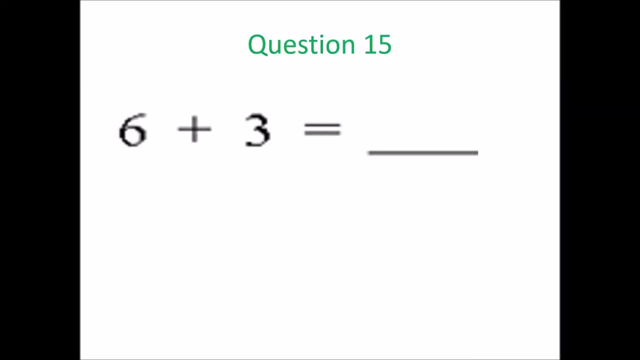 which one is it? wait on it. wait on it. what comes right after sunday, monday, question 15.. school grade two: six plus three. use your fingers. count on six plus three. use your fingers count on six plus three. use your fingers count on from six. count three one from six. yes, 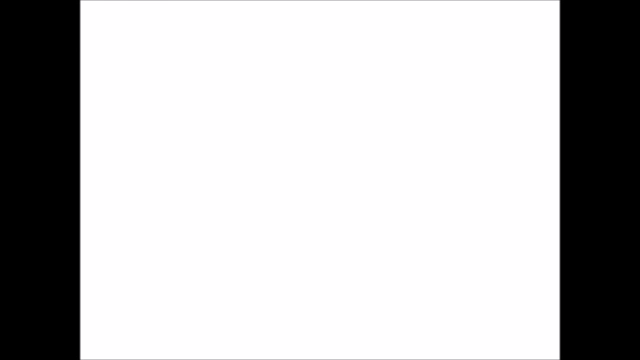 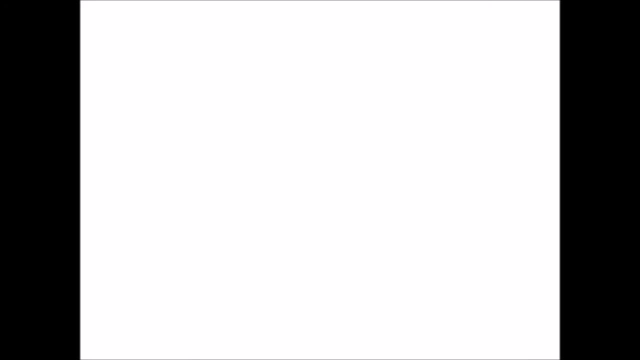 so what's the highest number? so what's the highest number? 15, then 10, 5 to 1. 15 then 10, 5 to 1. 15 then 10. 5 to 1, from the highest to the lowest descending, from the highest to the lowest descending. 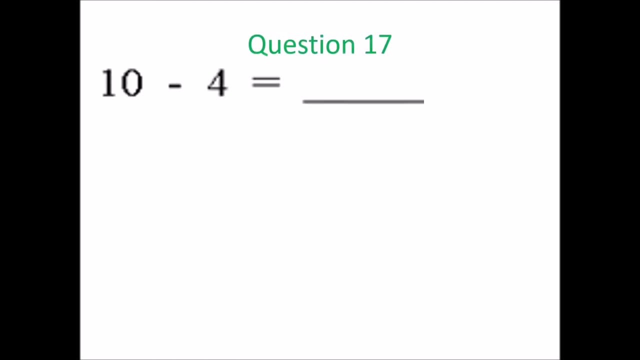 from the highest to the lowest, descending. it's going down, it's going down, it's going down. question 17: 10. take away four. question 17: 10: take away four. question 17: 10: take away four. use your fingers- ten fingers- take me. use your fingers, ten fingers, take me. 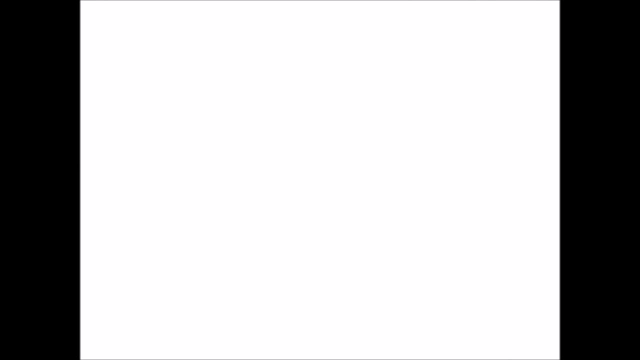 use your fingers, ten fingers, take me four, six, question 18.. question 18.. question 18.. here we go, grade two. here we go, grade two. here we go, grade two. circle the name of the month that circle the name of the month that circle the name of the month that comes right before march. 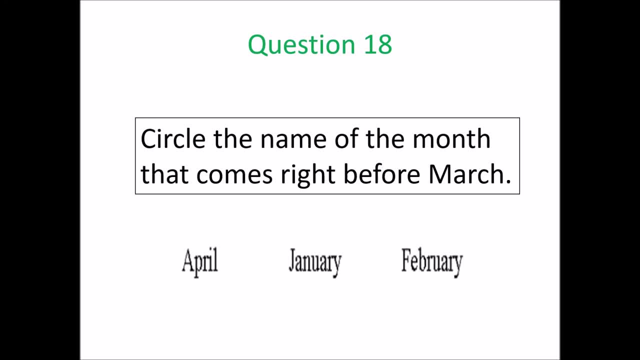 comes right before march, comes right before march. wait on it, wait on it. what comes right? wait on it, wait on it. what comes right, wait on it, wait on it. what comes right before march, before march, before march, february, february comes right before february, february comes right before. 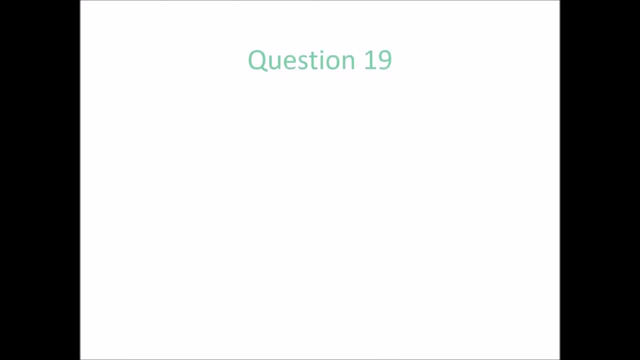 february. february comes right before march, march, march, question 19.. circle the letter on the third picture. circle the letter on the third picture. circle the letter on the third picture. the third picture would be the lighthouse. the third picture would be the lighthouse. 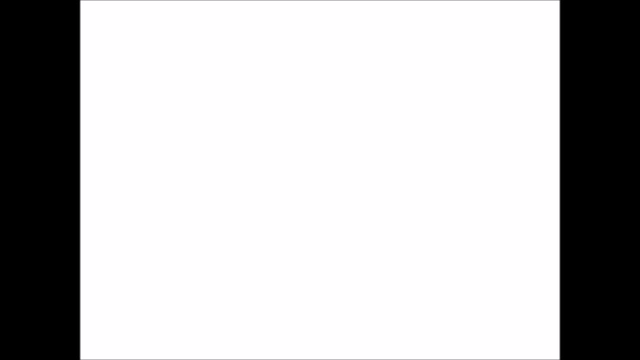 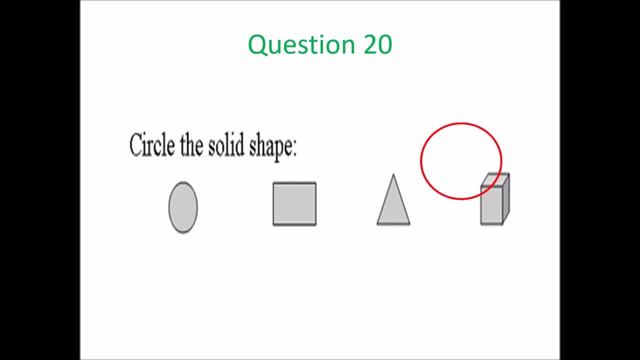 circle the solid shape, your plane, and circle the solid shape, your plane- and solid shapes. three of them are plain and solid shapes. three of them are plain and solid shapes. three of them are plain and one is solid. yes, it would be one is solid. yes, it would be. 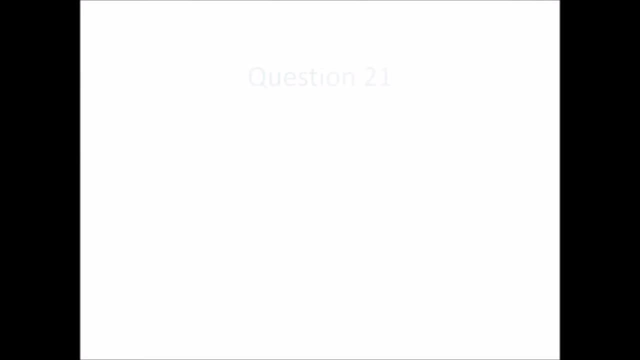 one is solid. yes, it would be the box shape at the end. the box shape at the end. the box shape at the end. it's a rectangular prism, question 21. it's a rectangular prism, question 21. it's a rectangular prism, question 21. you are adding 74 plus 12.. let's wait on. 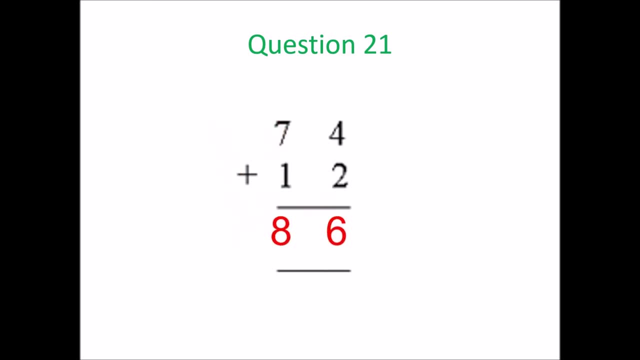 you are adding 74 plus 12.. let's wait on. you are adding 74 plus 12.. let's wait on it. add the four and the two. it add the four and the two. it add the four and the two and then add the seven and the one: 86. 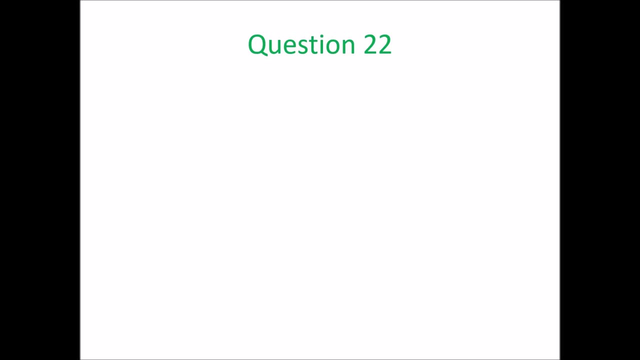 and then add the seven and the one 86 and then add the seven and the one 86. question 22: here we go. question 22, here we go. question 22, here we go. circle the cylinder, wait on it which one. circle the cylinder, wait on it, which one. 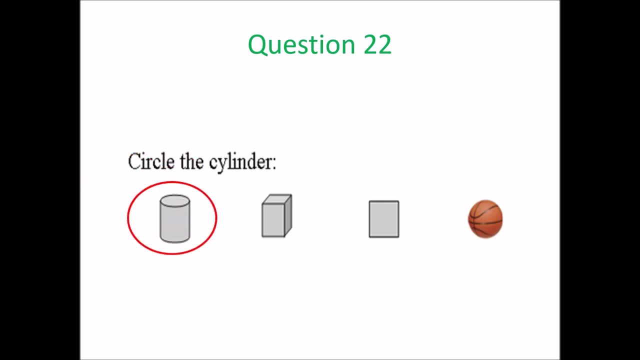 circle the cylinder. wait on it. which one is the cylinder? is the cylinder? is the cylinder the first one shaped like a can? that's the first one shaped like a can. that's the first one shaped like a can. that's the cylinder. very good, the cylinder, very good. 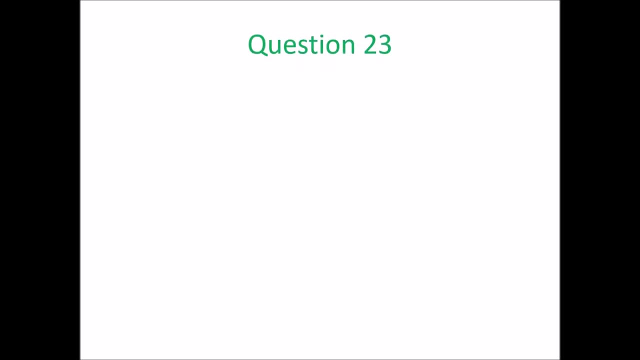 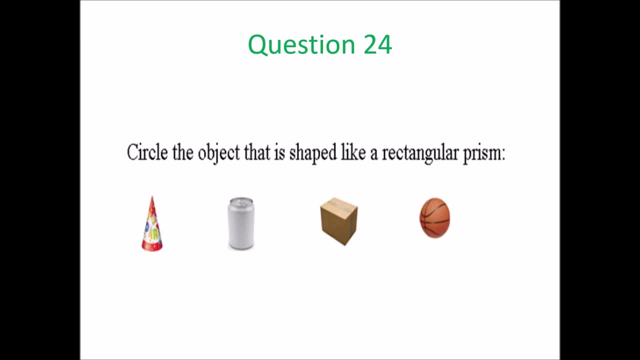 moving right along circle, the object moving right along circle, the object that is shaped like a rectangular prism. that is shaped like a rectangular prism. that is shaped like a rectangular prism. once it's shaped like a box, there it is. once it's shaped like a box, there it is. 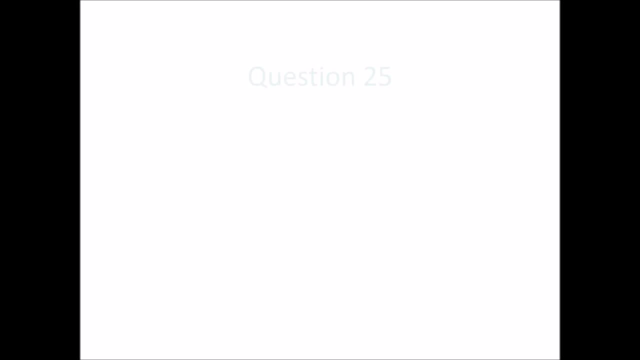 once it's shaped like a box. there it is. it's a rectangular prism. it's a rectangular prism. it's a rectangular prism. question 25: shade two quarters of the shape. so how shade two quarters of the shape? so how shade two quarters of the shape? so how much? 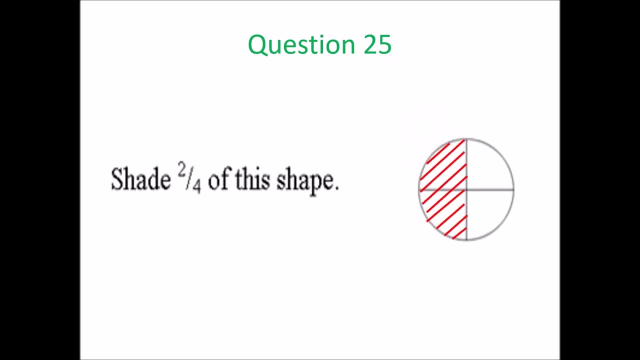 much, much. how much of the shape would you shade? how much of the shape would you shade? how much of the shape would you shade? you would shade two of those. so you get. you would shade two of those. so you get. you would shade two of those. so you get half of it, two quarters. 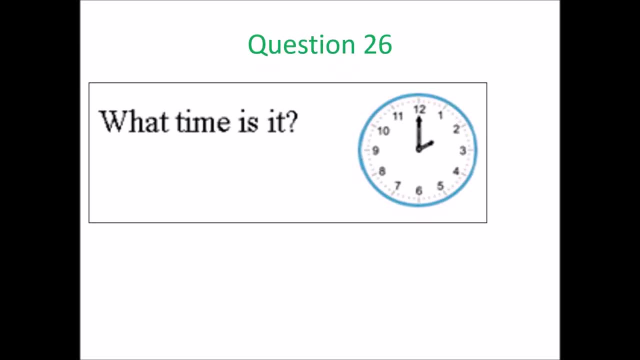 half of it, two quarters. half of it, two quarters. question 26: what time is it whatever? question 26. what time is it whatever? question 26. what time is it whatever the show on once it's on the longest on the show on once it's on the longest on. 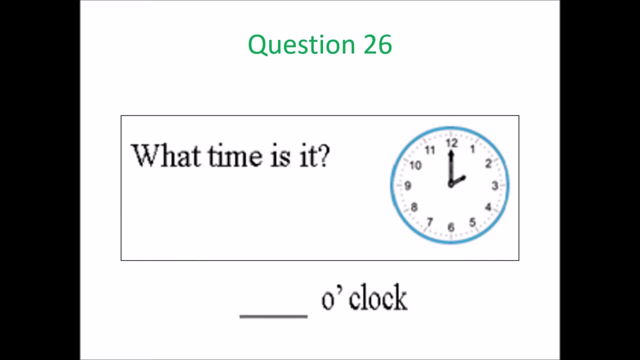 the show on once it's on the longest on 12th. whatever the show on points two- 12th. whatever the show on points two- 12th. whatever the show on points two. that's the time o'clock, so it is wait on. that's the time o'clock, so it is wait on. 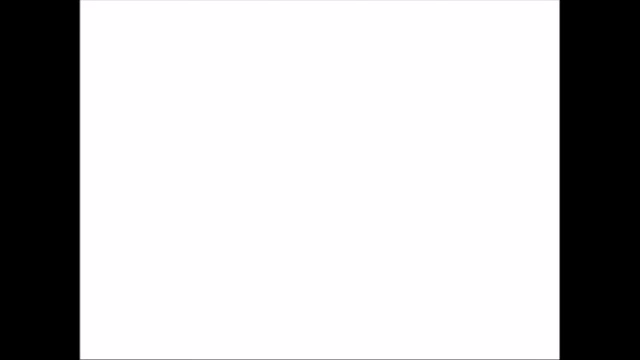 that's the time o'clock, so it is wait on it. two o'clock, it two o'clock, it two o'clock. question 27: that was easy. use the bar graph to answer the following. use the bar graph to answer the following. use the bar graph to answer the following question. and there is the bar graph. 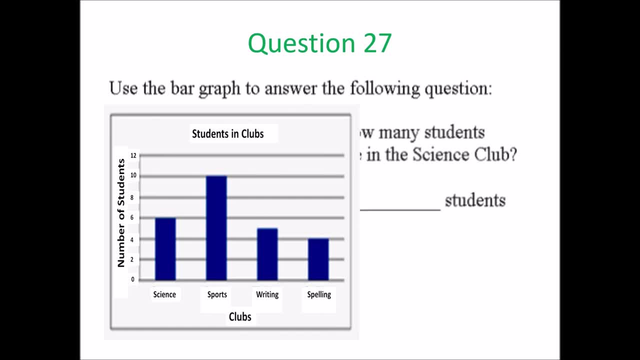 question and there is the bar graph question and there is the bar graph: students in the clubs, students in the clubs, students in the clubs- and you want to know how many students and you want to know how many students and you want to know how many students in the science club so find science. 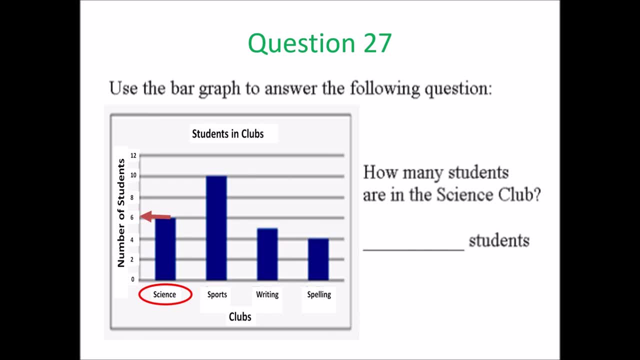 in the science club. so find science in the science club. so find science along the bottom and then see along the along the bottom and then see along the along the bottom and then see along the side what number it stops at side, what number it stops at side, what number it stops at. wait on it: six, six students.